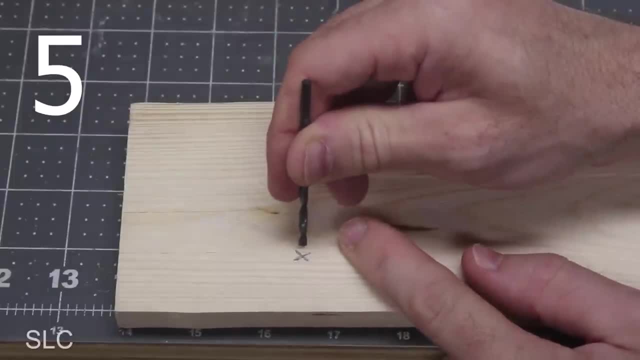 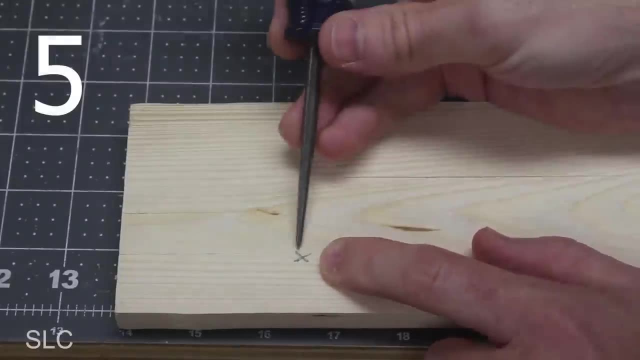 Now anytime you need to drill a hole with a drill bit, sometimes the drill bit is going to want to walk around before the hole actually starts And if you're trying to make an exact hole, then I'd suggest buying or marketing. So you're making yourself what they call an awl. 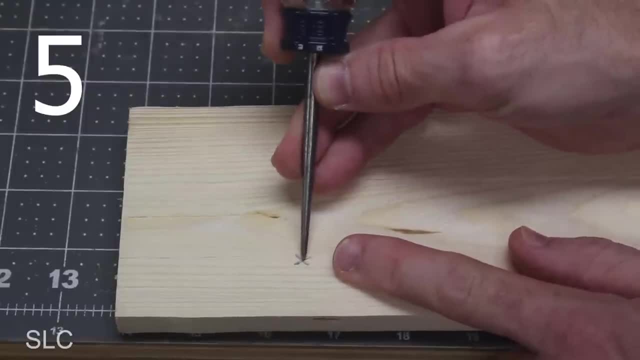 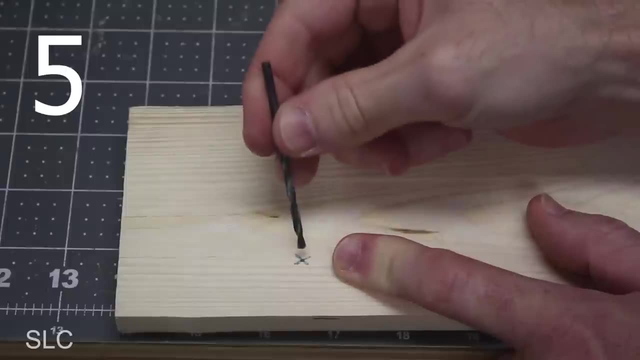 This right here is basically just a pointy piece of metal that will allow you to go in and get that same exact spot right in the middle and make a little divot And that way when you start it with your drill bit, it'll want to follow that divot and give you that exact spot. 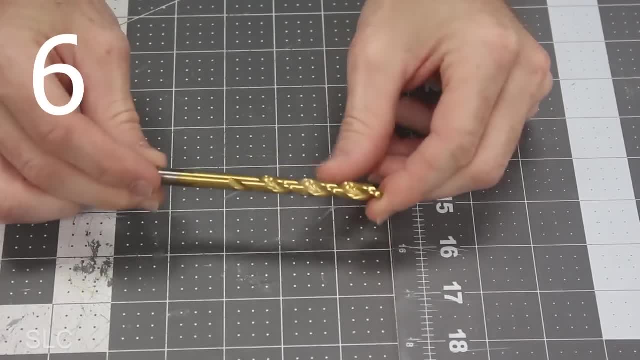 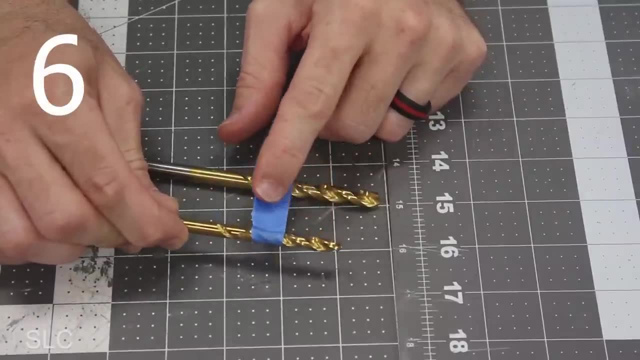 Now this next one is an oldie, but a goodie. Anytime you go to drill out a hole with a drill bit, it's sometimes hard to tell exactly how deep you're going to go. So in those cases, measure out exactly how deep you want your hole. put some blue painter's tape on there. 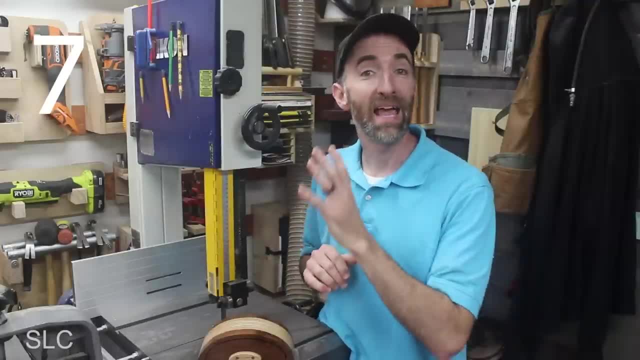 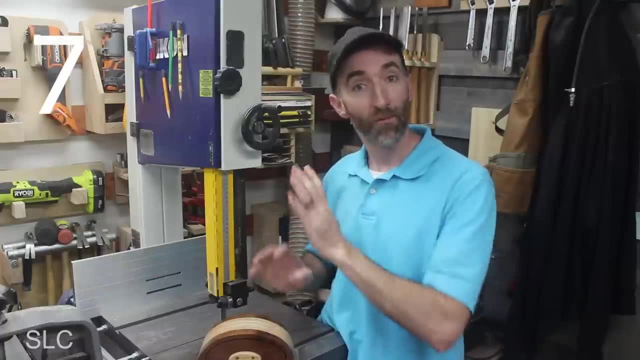 And that way you won't over drill. Now, anytime you're thinking about buying a new tool, especially if it's an expensive one, I strongly recommend taking a class or a course showing you exactly how to use it. For example, before I bought this bandsaw, I actually took a class and showed me how to make a bandsaw box. 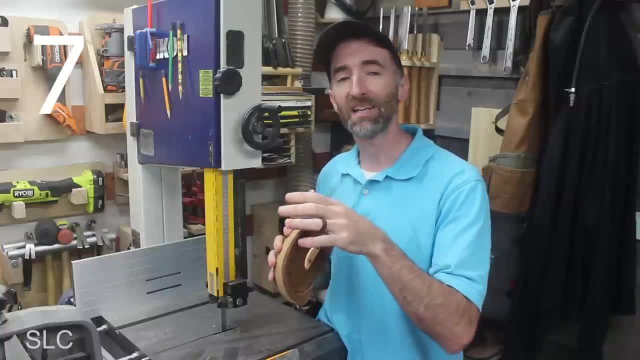 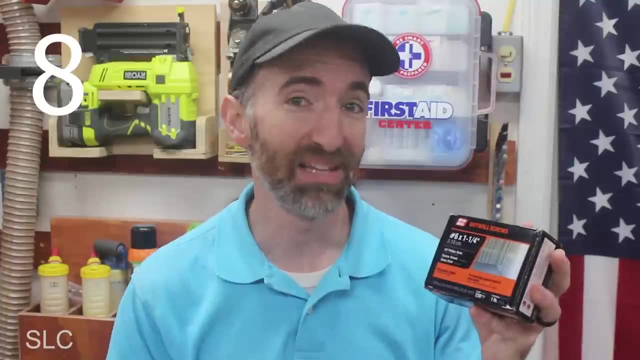 I learned a bunch from the instructor and he was there to show me exactly what I was doing wrong and how to correct it. So if you can afford it, try and take some classes. Now, this next one I am totally guilty of. When I first started woodworking is, I ran out and grabbed a bunch of tools. So this next one I am totally guilty of: When I first started woodworking is, I ran out and grabbed a bunch of tools. So if you can afford it, try and take some classes. So if you can afford it, try and take some classes. 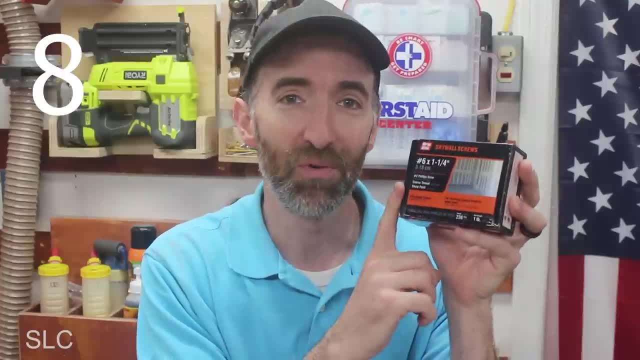 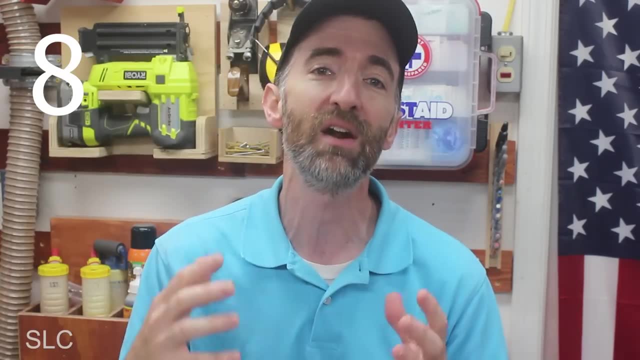 Now these are cheap screws. They're just drywall screws. These are horrible for woodworking. Usually they're really thin and narrow and are easy to break the head off, And now you have whatever's left is stuck in your wood and they're a big pain to get out. 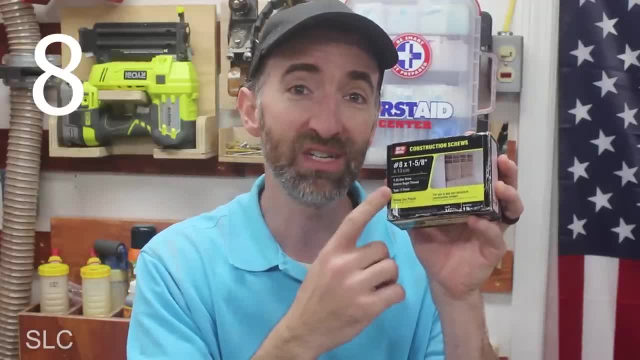 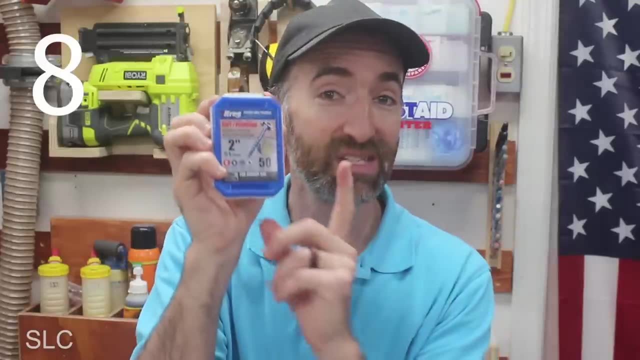 I'd strongly recommend, if you're going to use screws, to get some construction type screws, And those should help a lot better holding together and less likely to snap off the heads. Now, if you're going to use pocket holes, definitely get the appropriate pocket hole screws. 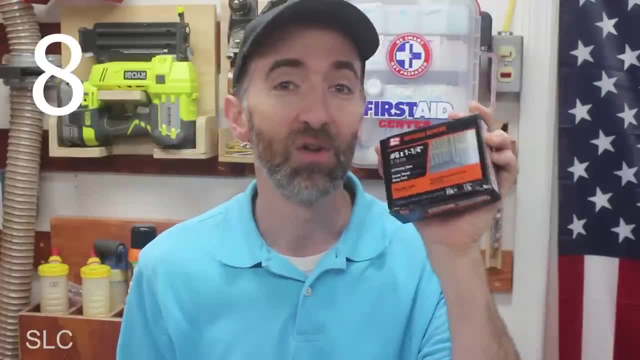 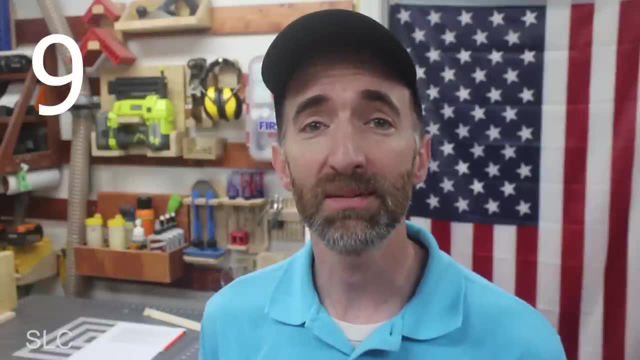 Do not use drywall screws for that. Do not use drywall screws for that. Now, if you ask a bunch of woodworkers what's one of the most important things to do when you're starting a project, A lot of them would tell you to make a plan. 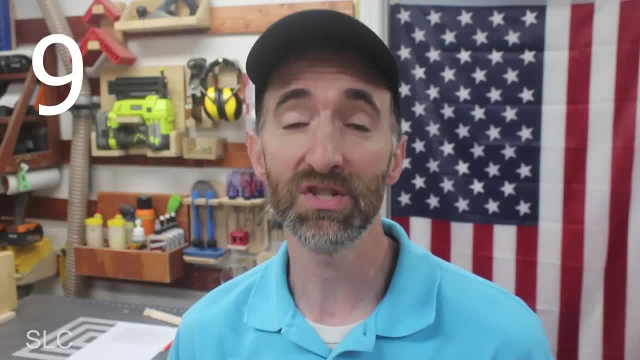 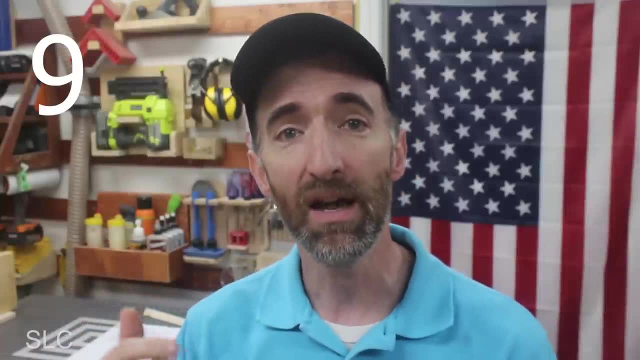 Now, of course, you don't have to make a fancy one like this. In fact, you could even order some online. In any case, you need to have something written out or drawn out So you know what the measurements are going to be and the angles you need to cut. 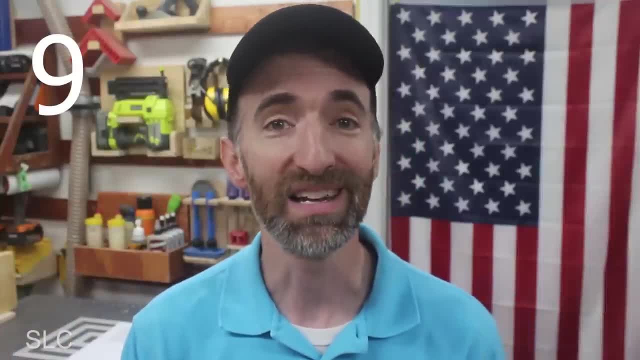 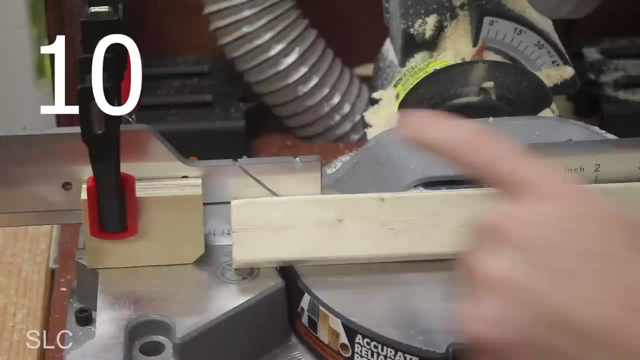 and so forth, to make sure that your project will be completed correctly. Because I guarantee you, if you don't have a plan and you run out in your shop and you just start making cuts, it won't look nearly as nice If, by chance, you need to make repeated cuts of the same length of a piece of wood. 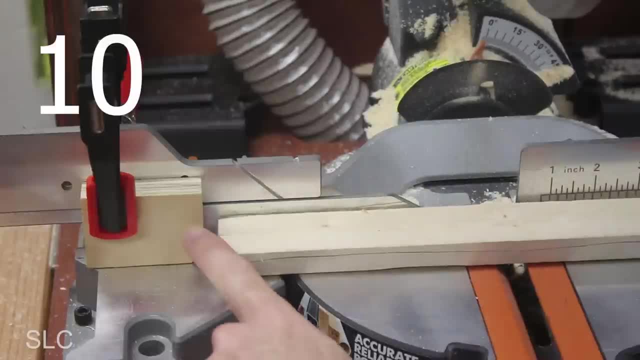 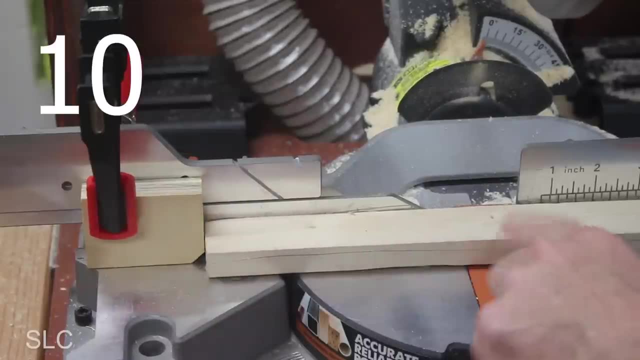 instead of going in and measuring out each piece and then making your cut, you need to set up a stop block. Basically, you need to find the exact length of the wood, set everything up and put a stop block here, And this allows you to make a cut, slide it in again. make a cut, slide it in again. 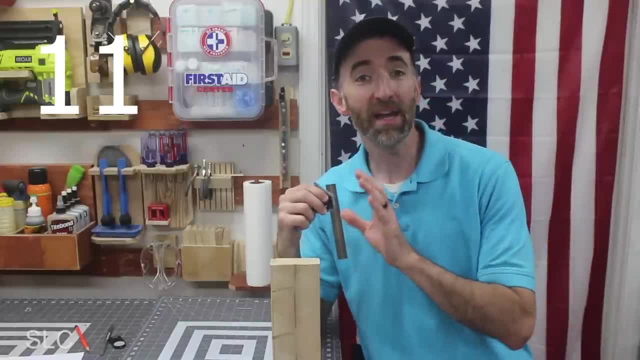 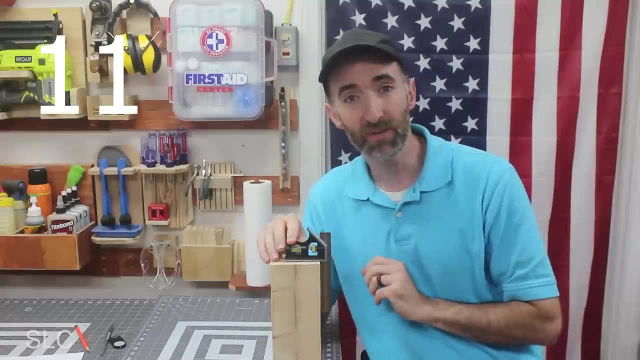 and you can do that over and over again real quick. Now, anytime you're buying lumber at your home improvement store, specifically if you need a really tight square edge, it's a good idea to double check the factory cuts Because in many cases they're not going to be square. 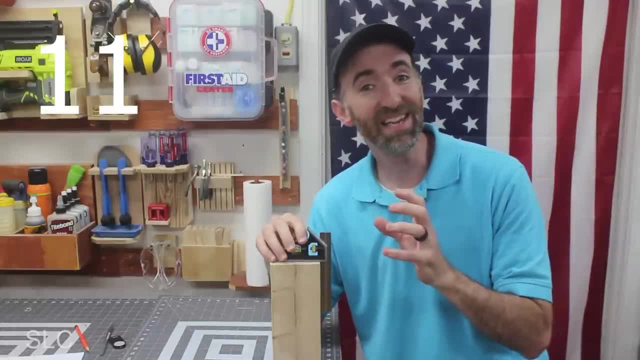 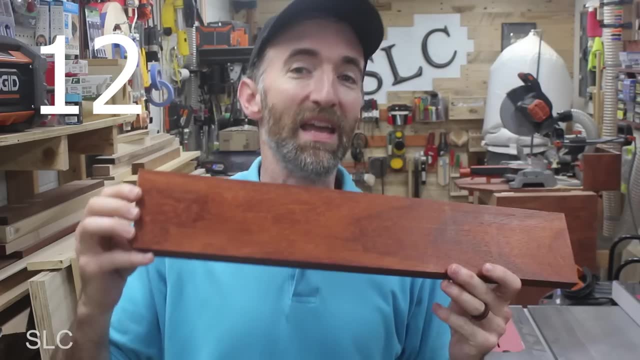 In this case it's almost dead on, But in many cases this right here will actually be a few degrees off and thus throwing your angle of whatever you're making a little bit off as well Anytime you store wood in your workshop. just keep in mind. 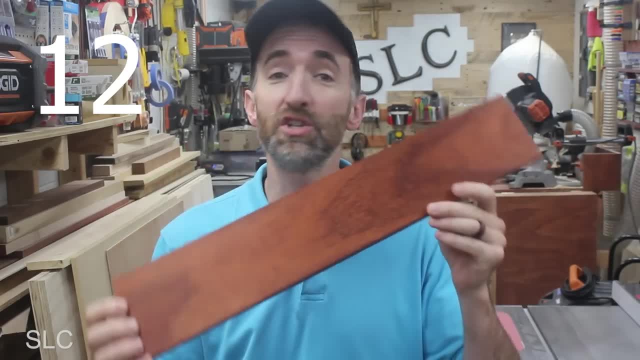 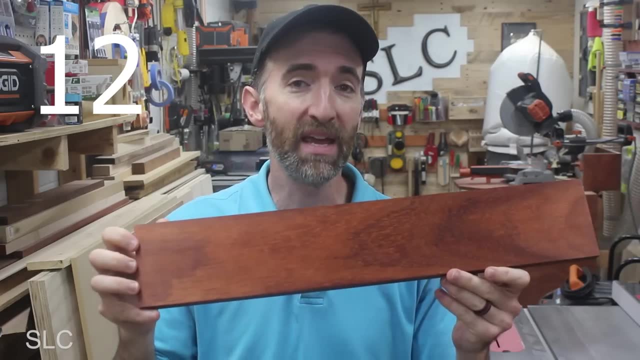 as temperature changes and humidity changes, the wood is going to change as well. So if you're going to work with a piece of wood and try and make it really flat and then you're going to actually leave it in your shop for a couple days, 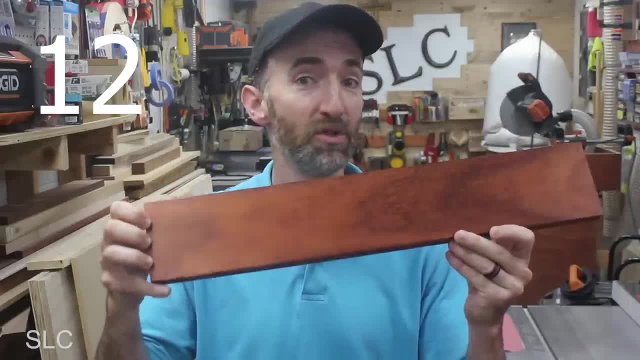 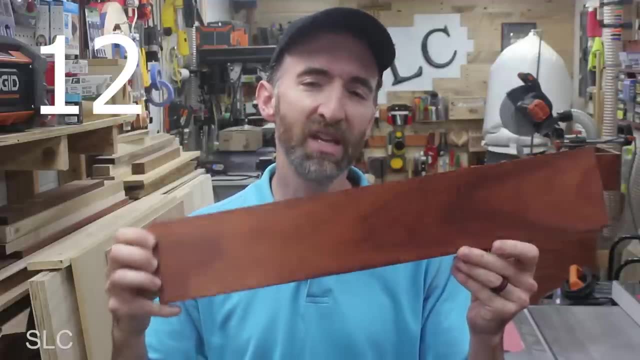 when you come back, there's a good chance. it may have slightly warped or just changed shape in general. So go back, double check all your measurements, Because if you're not going to put it together in one day, there's a very good chance. 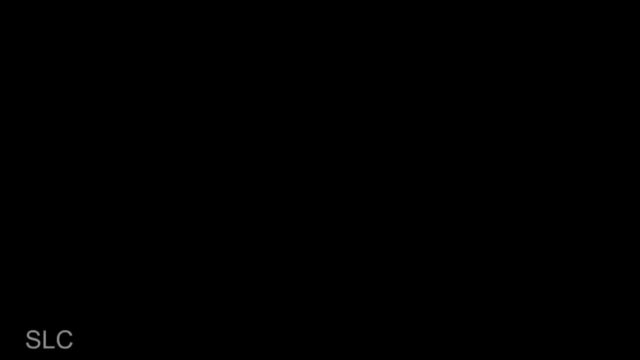 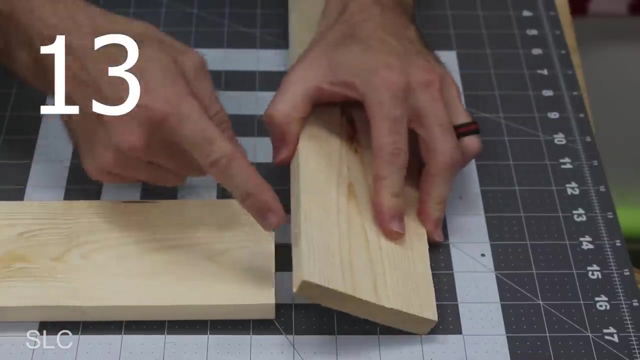 it might cause a little bit of an irritation when you're trying to put it together later. Anytime you're trying to connect two pieces of wood together, especially if it's side grain to end grain, here it's a good idea to avoid just using glue. 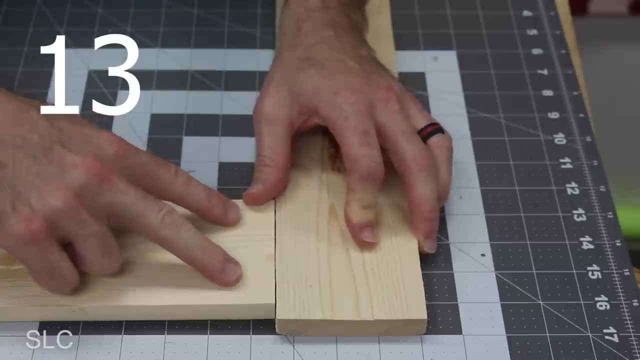 You want something in addition to that, So in my case I would maybe use some pocket screws or some other type of joinery to make sure those stay together. Otherwise, over time, you're going to end up with a piece of wood. that's going to be. 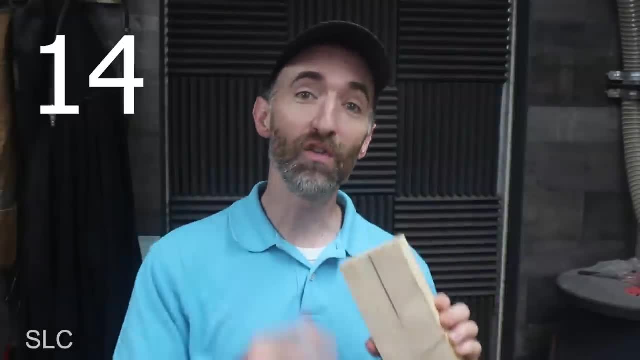 a little bit smaller than the size of your home improvement store. If you're just starting out woodworking and you head over to your local home improvement store when you're looking at the 2x4s, please remember that when it says 2x4s. 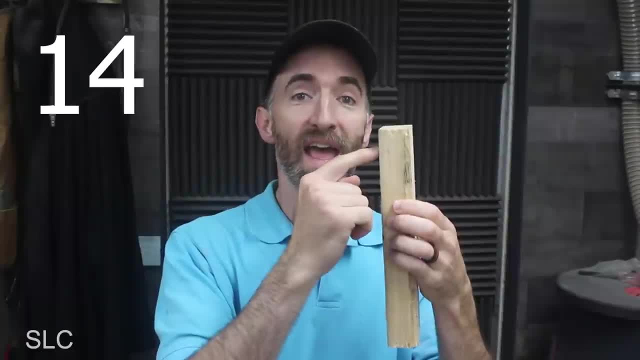 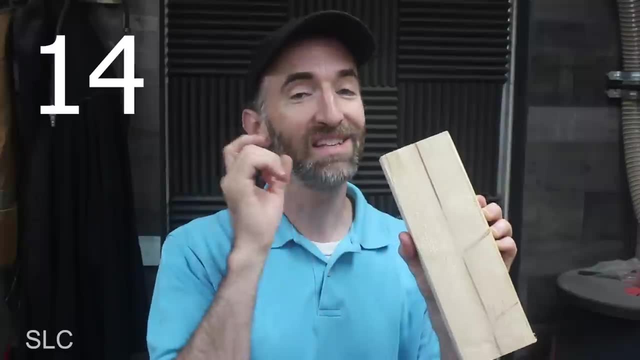 it's not a 2x4 dimension. It's actually 1.5 by 3.5.. Now there's a whole history lesson on exactly why this is the case, but just remember that when it's a 2x4, it's a little bit smaller. 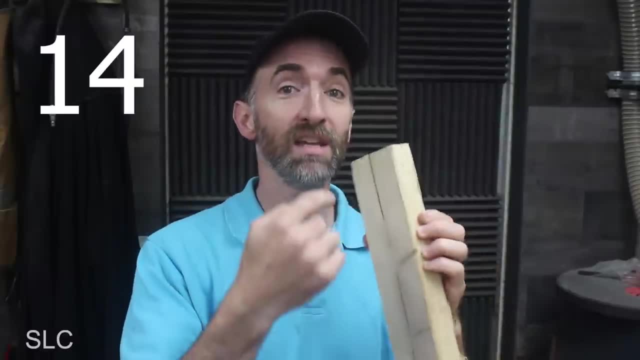 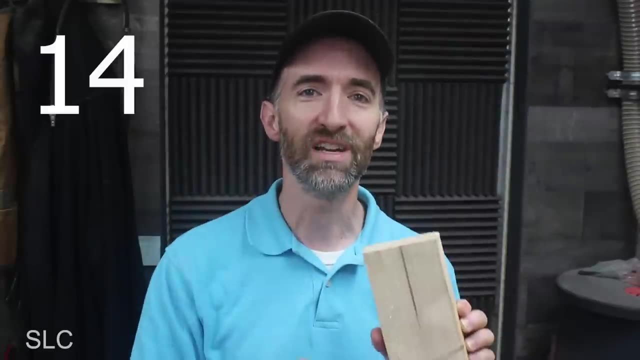 Now, if you're dealing with hardwoods, there's a very good chance that when they say it's 2 inches and 4 inches, it will be 2 inches and 4 inches. But in either case, take a measure tape with you so you know exactly what you're looking at. 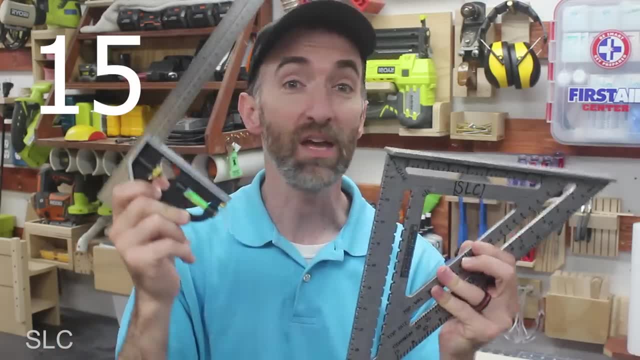 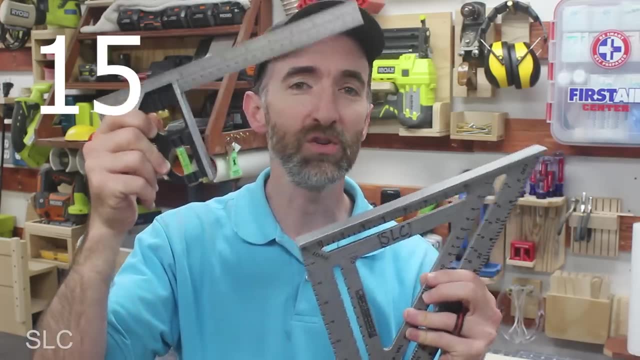 Now, anytime you buy any type of squares or any tools to make sure that your projects are nice and straight, you need to recalibrate these and make sure they are correct. I don't care if they're the cheap version or the high top end stuff. 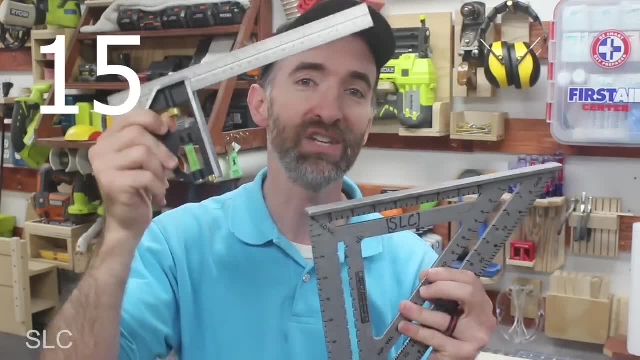 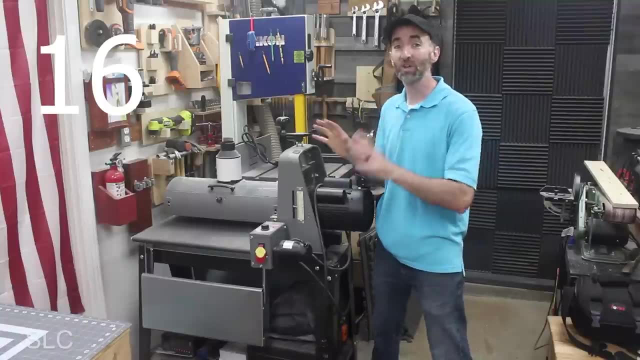 In the process of them getting from the factory to your hands. there's a very good chance they were knocked out of position and you need to make sure these are square so that your projects will end up as square as well. Now, over time, your workshop is going. 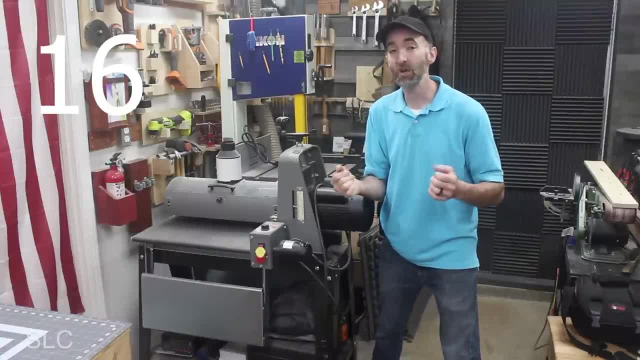 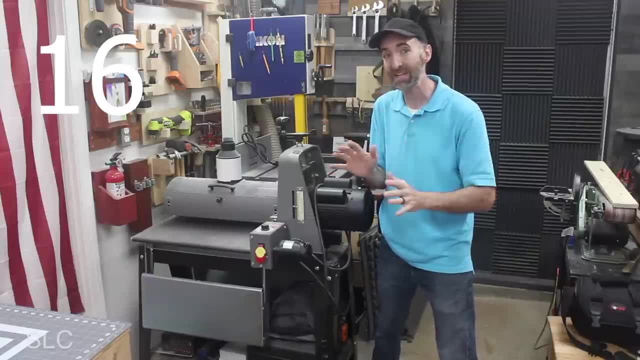 to continue to grow And if you have a small shop, like I do, I highly recommend putting all of your tools and your cabinets and your workbenches on some type of rolling system or casters, For example. I currently have three tools set right here in this corner. 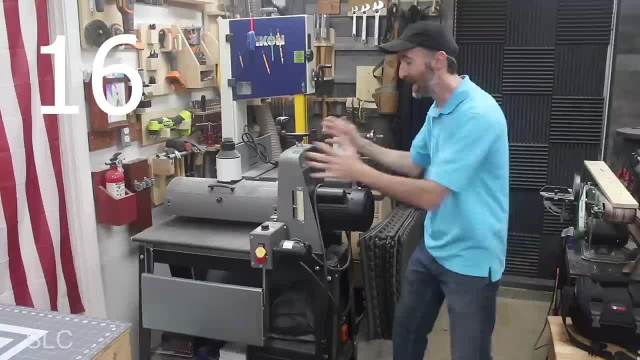 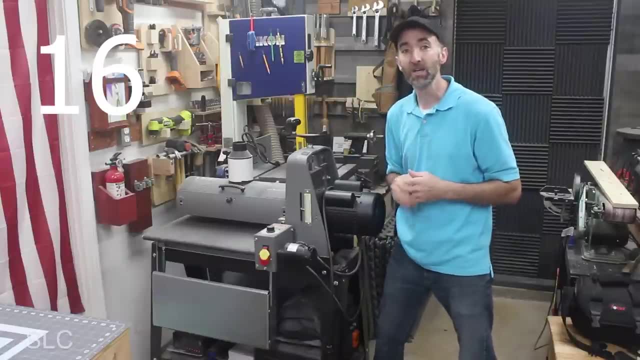 In this current position they're not usable. But because I have them on casters, I can easily move them into an area that I can easily work with them or just get to the one behind it. So I highly recommend putting them on some type of a rolling system. 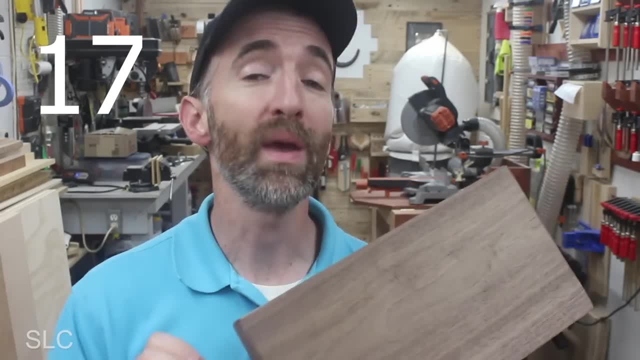 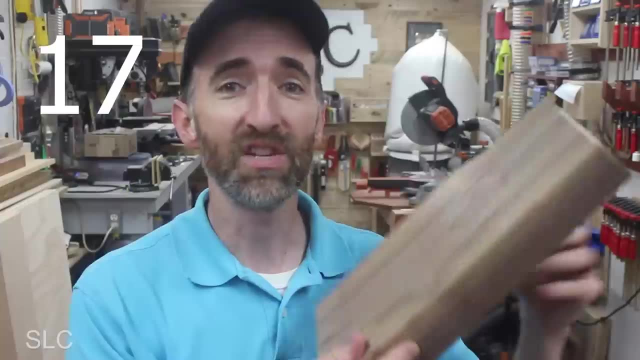 Now, anytime you're about to build a project, I strongly recommend you going out and actually purchasing the wood. Get your hands on it so you know exactly what you're purchasing, Because I guarantee you that if you have some delivered, they're not going to pay nearly as 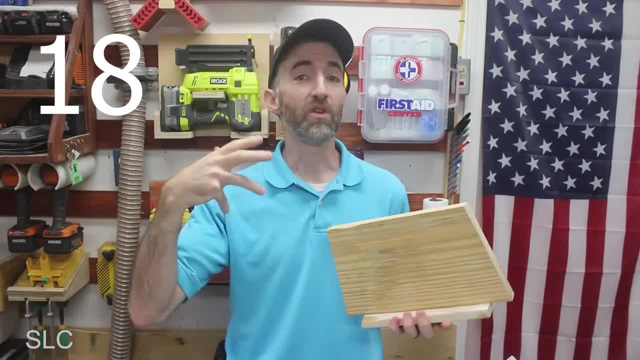 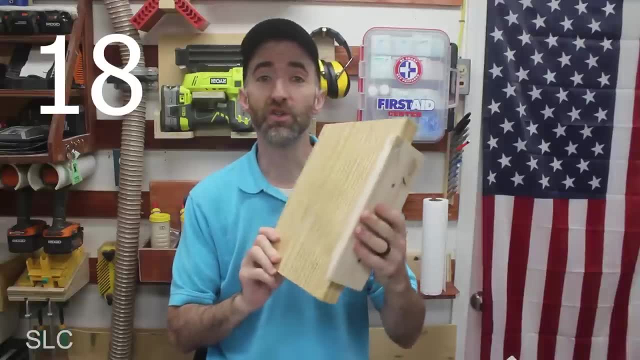 much attention to the quality of the wood. Jigs are very important whenever you're making repeated cuts, And I strongly suggest making any jigs that you can use over and over again. For example, this right here is super simplistic, but it's a jig I just recently built. 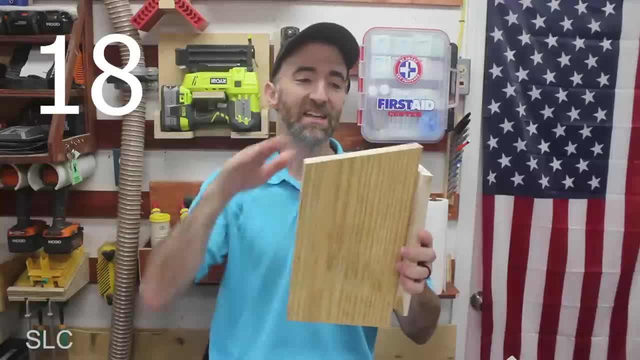 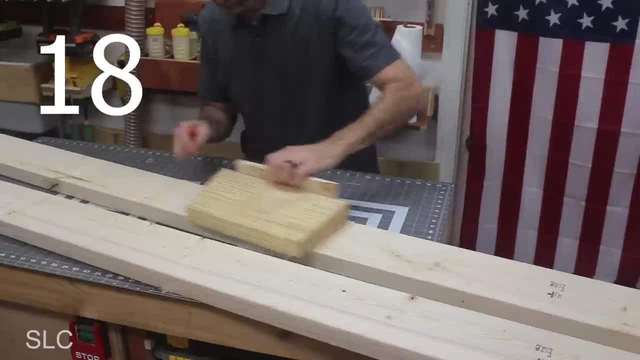 a ladder for my back building here and I needed exactly 15 degrees all along the side rails. Well, instead of me measuring them over and over and over again, I had a line go up, had a line and go up. In fact, 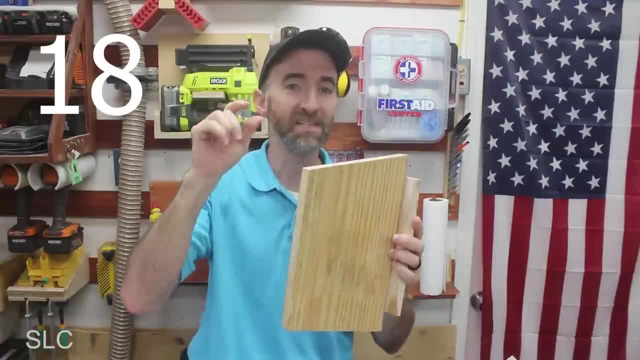 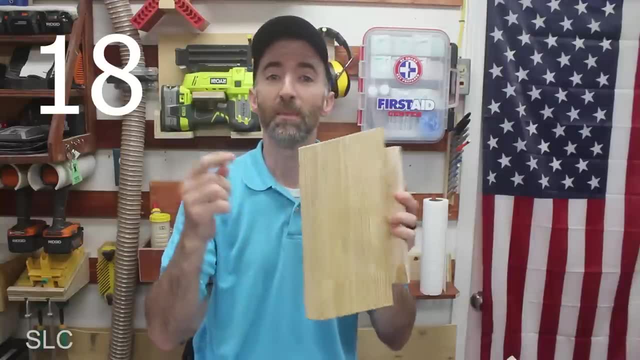 this right here actually saved me, because I goofed up a little bit on the lines and I was able to go back and repeat those exactly where I needed them without having to remeasure several times. So remember, jigs are important and they don't have to be super fancy. 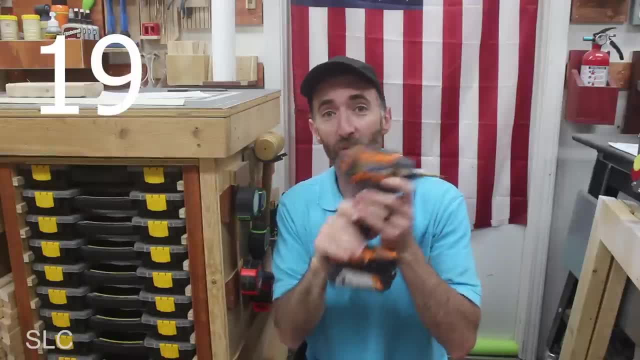 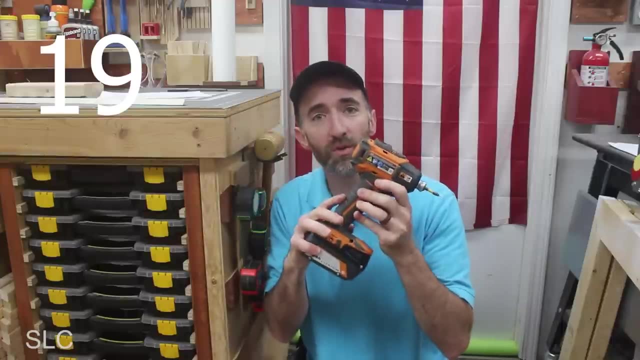 There's a big debate in the woodworking world of what do you do first, collect tools or build yourself a workbench? Now I would suggest holding off on your workbench just for a little while and start using tools to build. The reason why is you'll quickly learn exactly what kind of accessories you would like on your 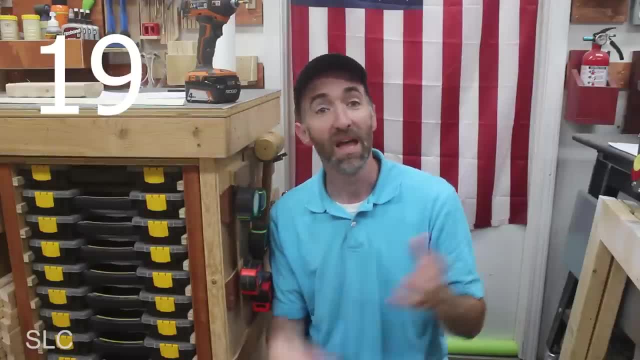 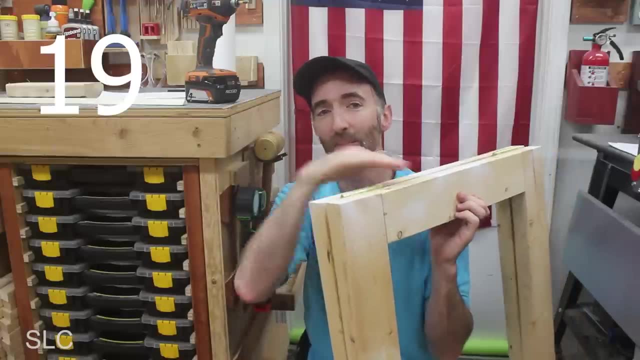 workbench. So when you do build it, you can incorporate that into it. Now, if you need a temporary workbench, I'd suggest going out and building yourself just a couple of saw horses. Then you could just put a piece of plywood or some MDF on top of it and use that as your workbench. 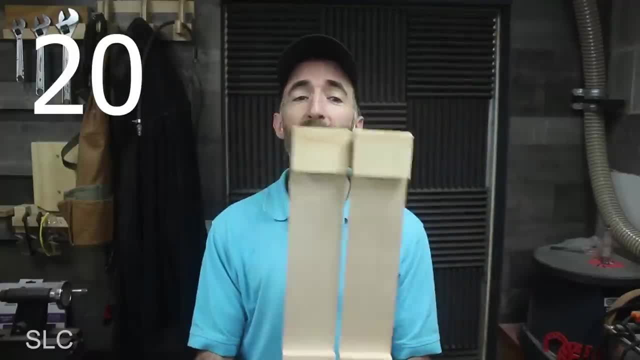 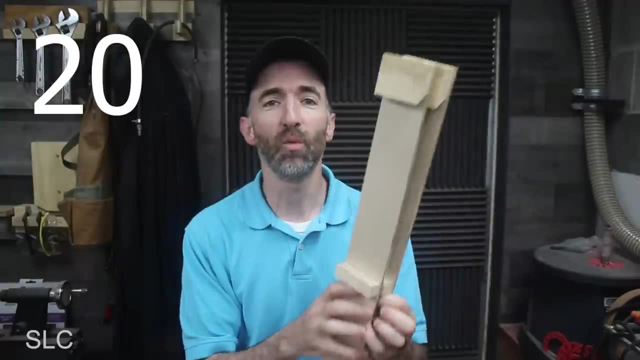 Anytime you're making two of the same exact piece. if you can try and make it extra wide and then just cut it in half on the table saw, This will allow you to have two pieces that are exactly the same. You don't have to worry about the size of the table saw. You don't have to worry about the 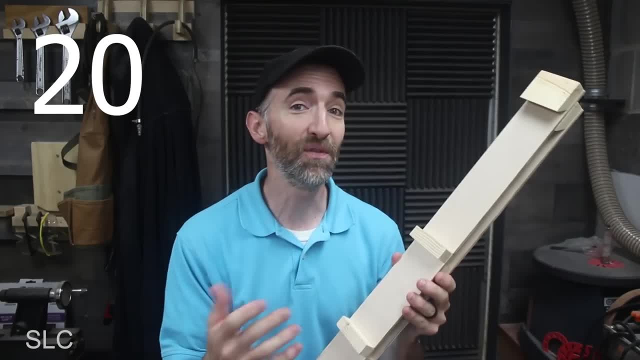 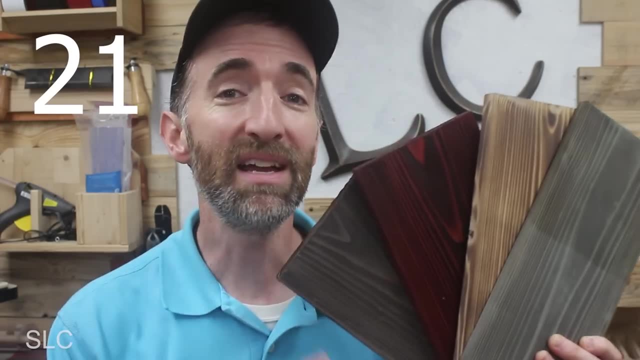 bottom being a little bit off if you make them separate. I sometimes still forget this. In fact, when I was making this project, I was reminded: hey, why didn't you just make it extra wide? So don't forget that Now if you're planning on staining your project or just even adding a. 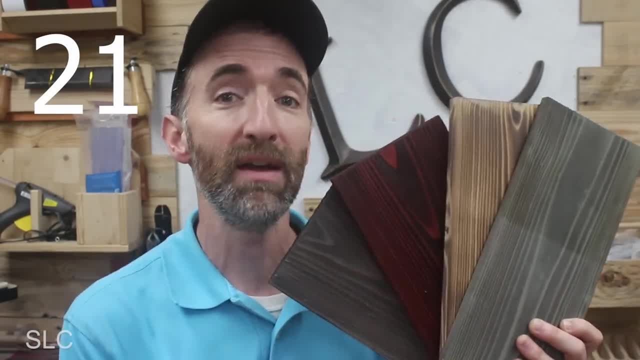 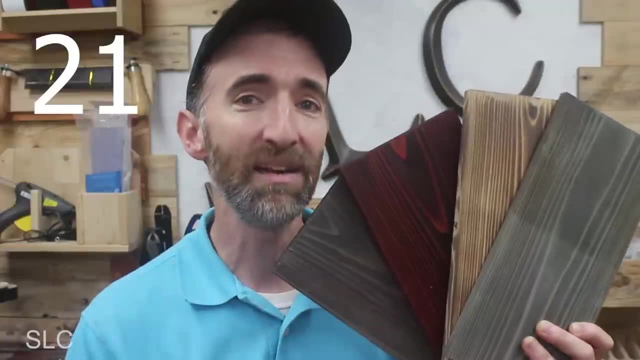 finish to it. I highly recommend going and get some of the scrap leftovers so that you can test out the stain you're thinking about, Because I guarantee you some of these colors will look completely different on different types of wood. So test it out so you don't regret it later. 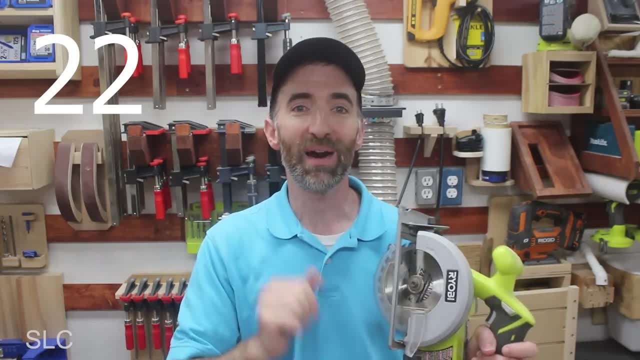 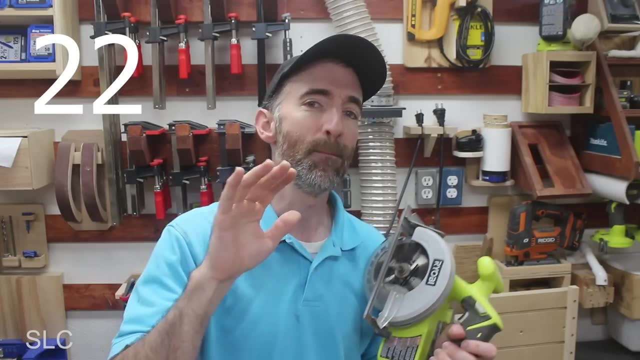 So what's more important? buying some bunch of tools at the low end price and just have them break occasionally, or saving up and waiting a long time to buy the high end tools? I actually believe there is a middle ground for that. 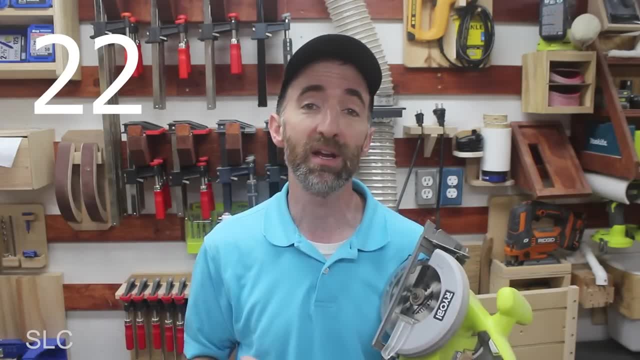 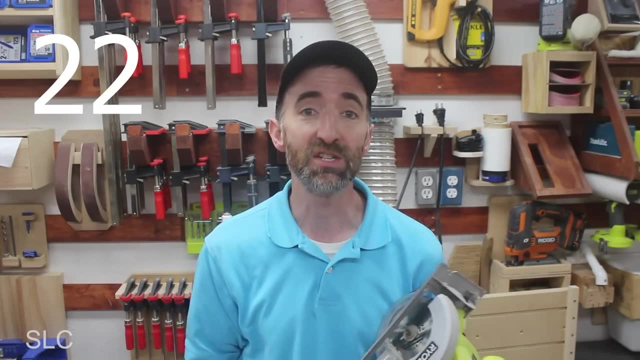 When you're first starting out, especially if you don't have a lot of spare money to spend. I recommend buying some of the more basic lower end tools, Because this is something you're just going to be using on occasion. Now, if you start using these on a regular basis and you figure out, 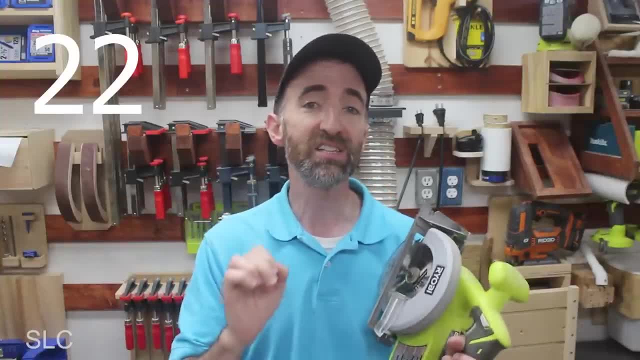 exactly what you want to do and you really love woodworking, then I'd suggest start to save up for the higher end tools, For example. if you're going to be using a lot of woodworking, you're going to want to keep any of your tools, with your tool accessories, For example. I have a high end table. 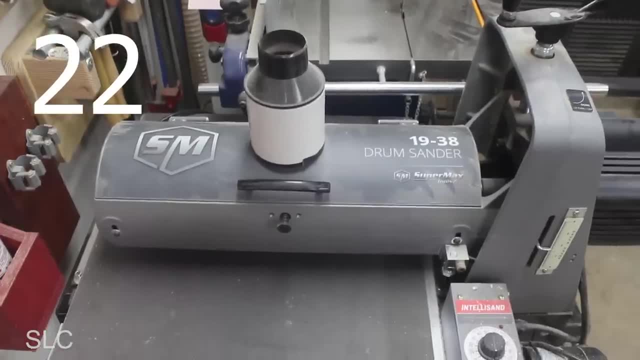 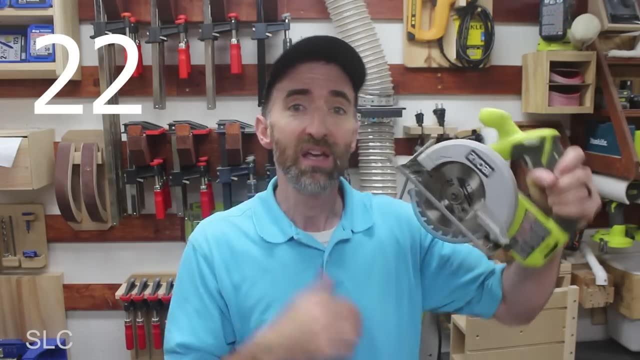 saw. I have a high end band saw and drum sander because I knew I was going to be woodworking for a long time, But I also have a combination of some of the lower tools that I started out with, So just keep in mind that you don't have to initially buy top end tools. 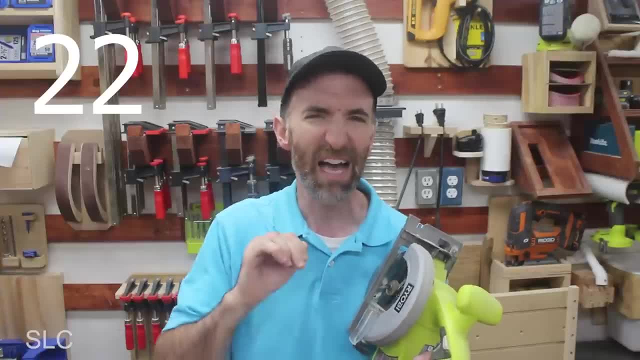 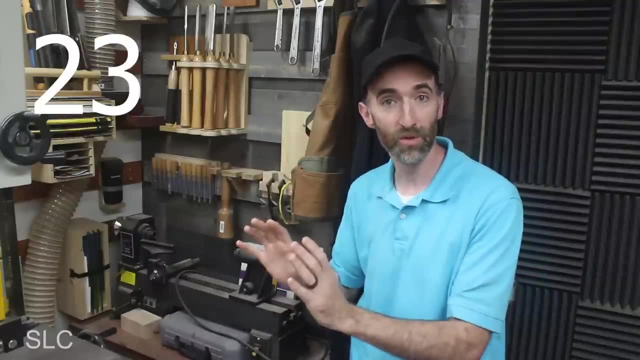 but if you're going to be doing this for a long time and you know you like woodworking, I'd definitely suggest saving up for them. Now, when you're starting off your workshop, it's very important to remember you need to keep any of your tools with your tool accessories. 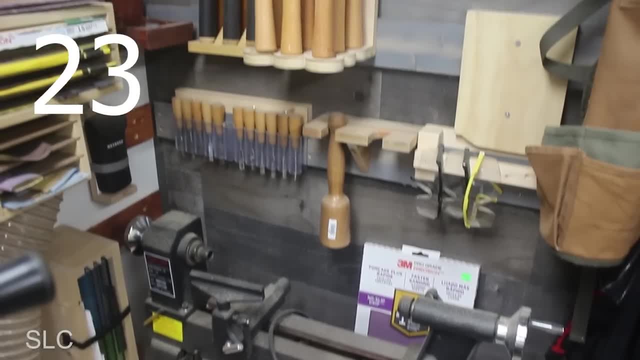 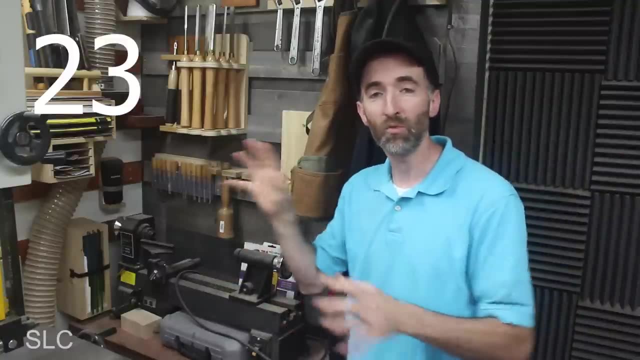 For example, right here is my lathe and right above it is where I have some of the tools for carving. Now, if I had this on a different wall in my shop or in a drawer somewhere, it'd be challenging because I'd have to run around and grab stuff, wasting time. 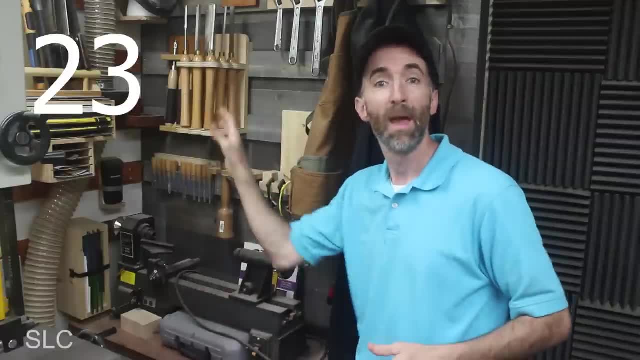 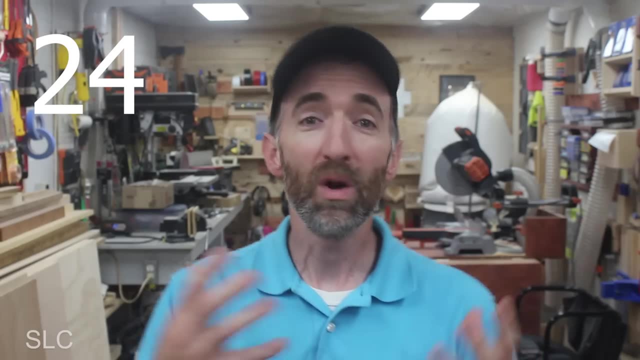 potentially falling over or getting hurt with one of the tools, But as long as it's within arm's reach, I can grab it, use it, put it back and use something else. Remember: tool organization is very important, One of the things I highly recommend in a 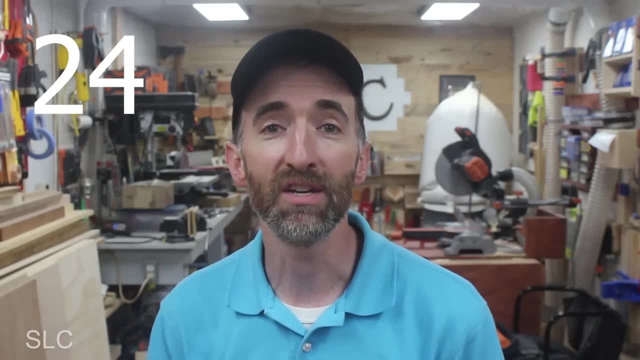 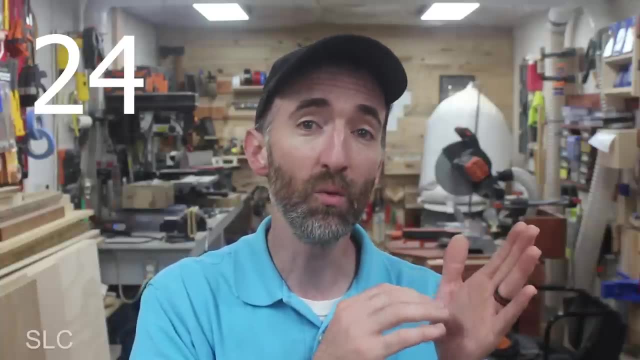 workshop is good quality lighting so you can see everything that's going on in a shop. That way, it's less likely for you to make mistakes or even get injuries. Plus, it'll give you a chance to see the true color of your wood. 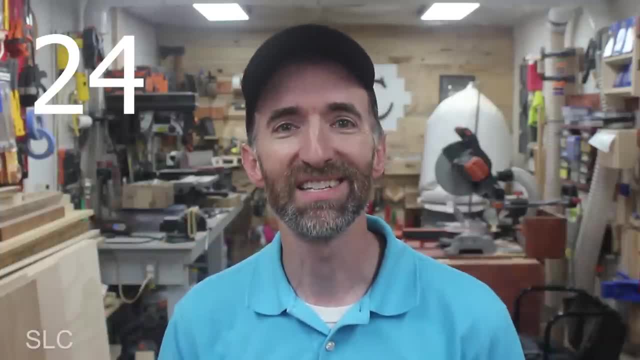 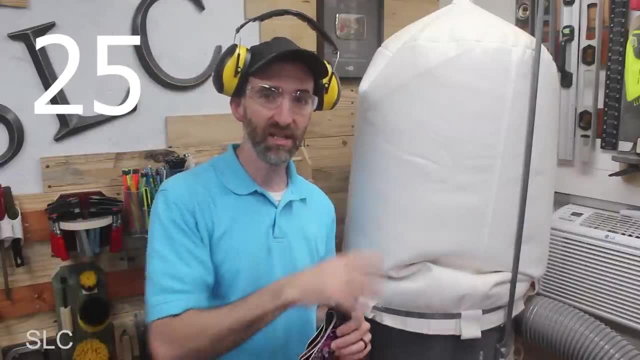 and any stains you might be applying. So make sure you get some good quality lights. And, of course, a woodworking video isn't complete unless I mention safety equipment, which is eye protection, ear protection and some dust collection equipment. If you don't. 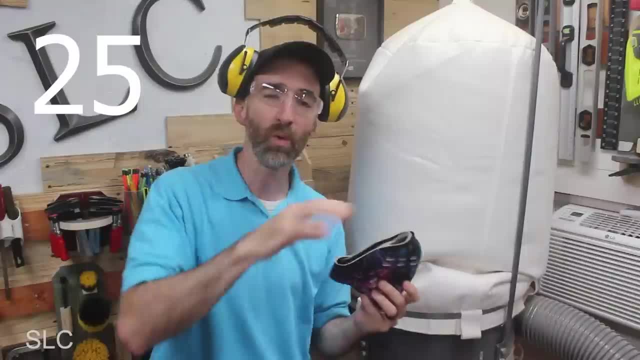 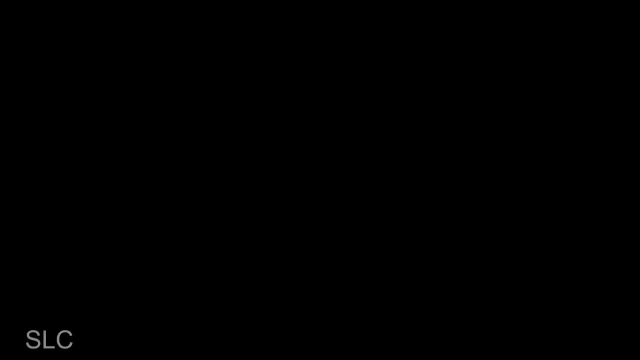 by chance have dust collection. make sure you get an appropriate mask that you can wear whenever you're working in your shop so you don't breathe in all those small particles. And if you're just doing a Japanese or Chinese shootout, make sure you have a. portable napkin. I mean, it's aён one, but it's just a little bit of a hassle. It only takes a couple of weeks to make one hundred and twenty miles of footage. So there is going to be a range of different types of filmowners out there that are going. to be offering this if you're doing a woodworking project, but since you're using this as a camera, we're not going to get into. you have to give it a little bit of time. So I hope that you guys are spending some time with us and have a great week. Thanks for watching. So I'm going to be back around in a moment, but I will keep you posted on the external comments and things like that. I'll be back in a few minutes. Thanks, 407 0000.. I'll see you later. Hashtag: 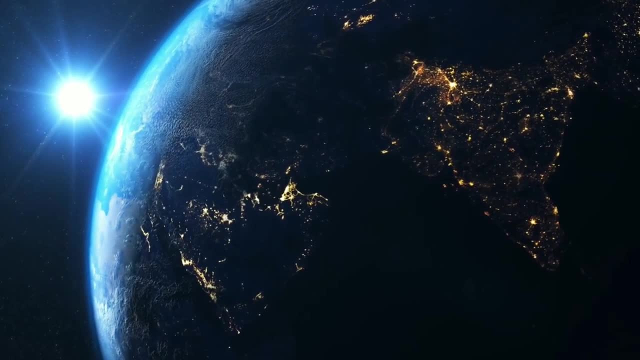 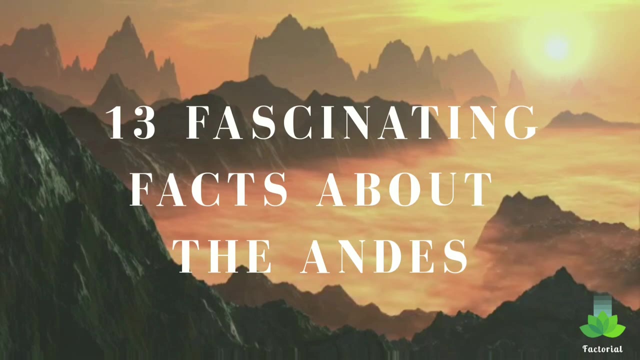 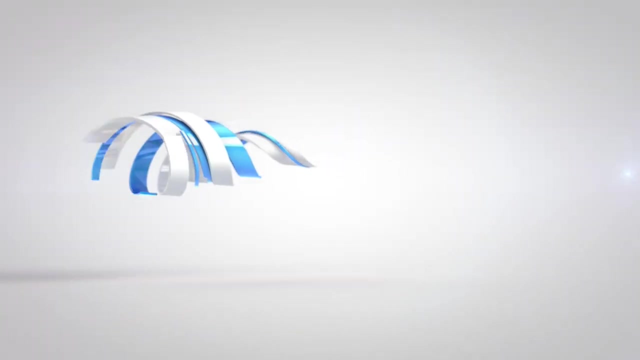 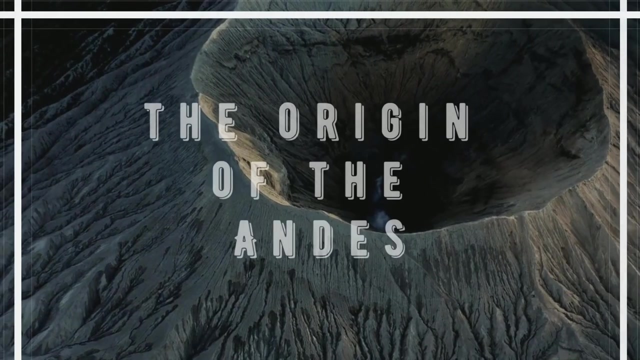 Hello everyone, I am Samik. Welcome to Factorial. Today, I am going to tell you some fascinating facts about the Andes. So, without wasting your time, let's get started. The origin of the Andes: The Andes mountain were created over 50 million. 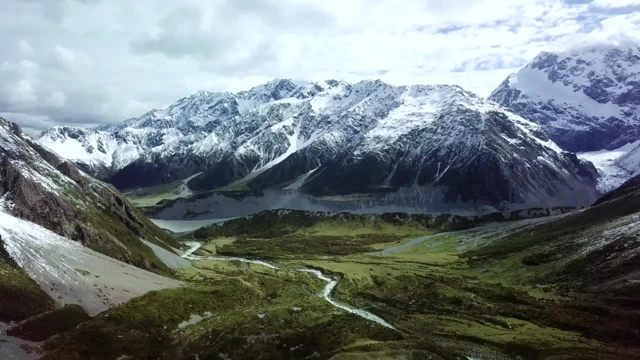 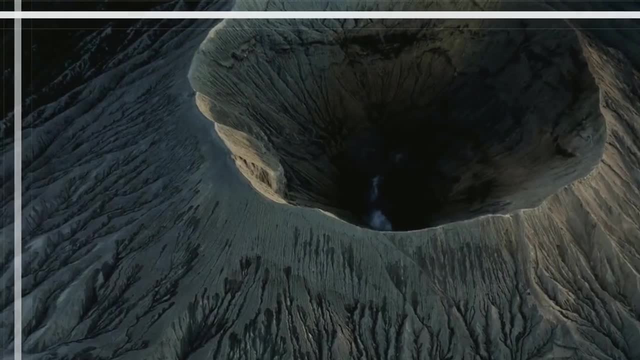 years ago, when the South American and Pacific tectonic plates collided. It is a collection of numerous mountain chains which joined together in what are called orographic knots. The etymology of the word Andes. The etymology of the word Andes has not been.